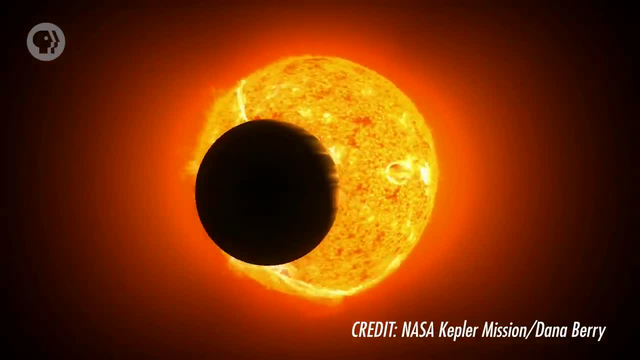 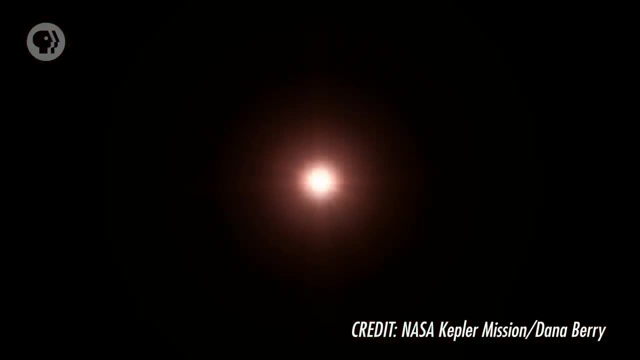 The biggest problem is any such planets would be faint, far away and sitting right on top of their parent star. Being able to see one in a telescope would be like trying to spot a firefly sitting next to a searchlight. So if you can't spot a planet like that directly, 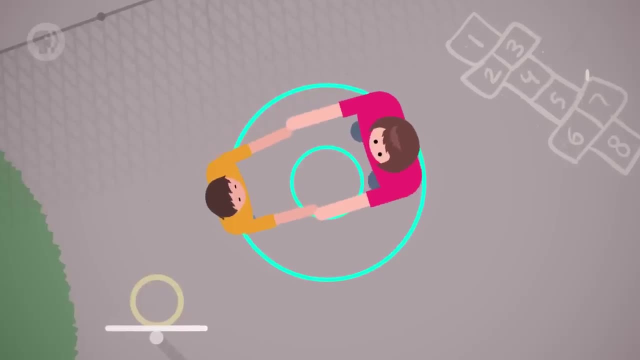 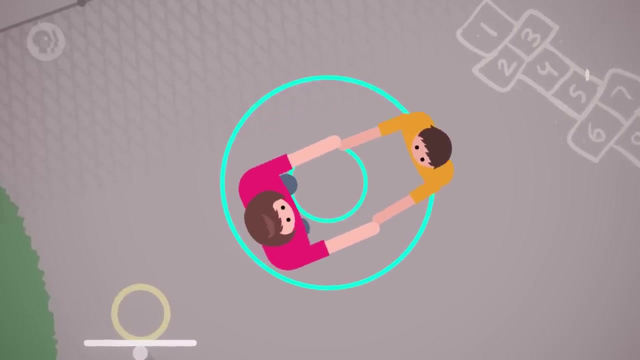 maybe you can spot it indirectly. Imagine two kids, one big and one small, facing each other. They clasp hands and start to spin around As they do. the little kid who weighs less will make a big circle and the 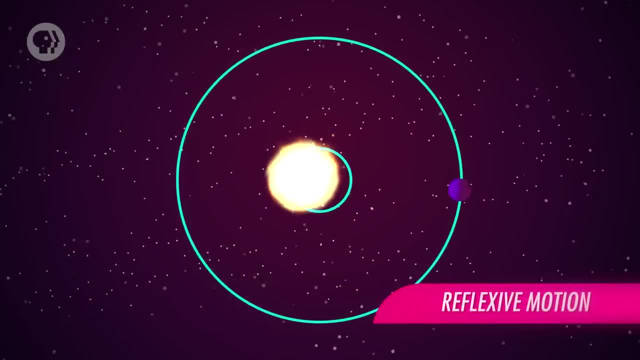 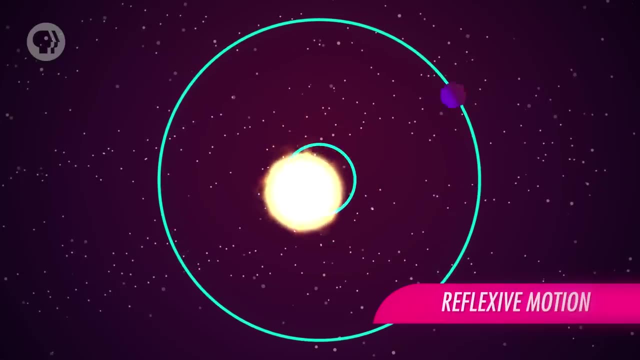 bigger kid will make a small circle. The same would be true of a star and planet. As the planet orbits the star, it makes a big circle or ellipse. But the planet has gravity too, and it tugs on the star. That 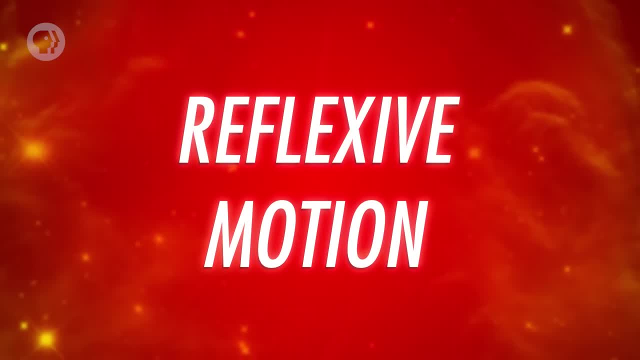 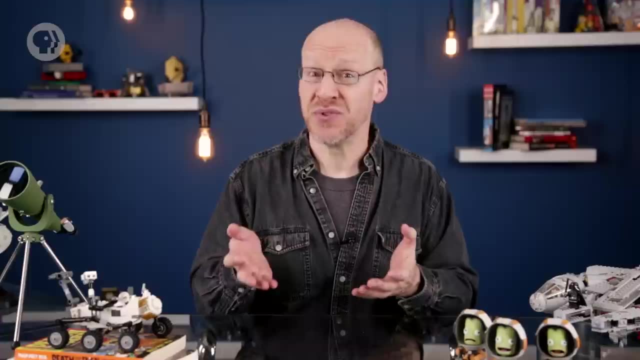 means the star will make a small circle, what's called reflexive motion. For a long time astronomers looked really hard for this motion in nearby stars, But it turns out that indirect effect is also too small to see. There were a few false alarms, but no real planets. Then, in 1992, everything changed. Astronomers Alexander Volshan and Dale Frail made a shocking announcement: They found not just one planet, but two orbiting a pulsar, the dead remnant of a star that had exploded. 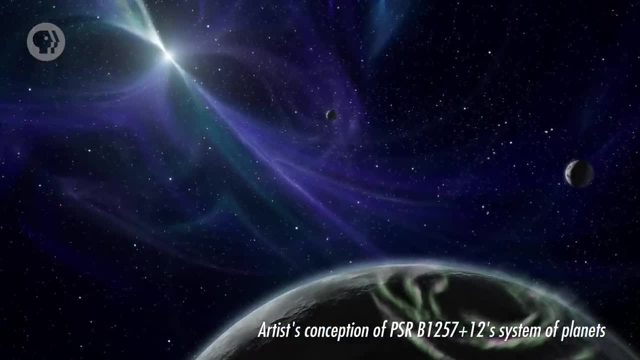 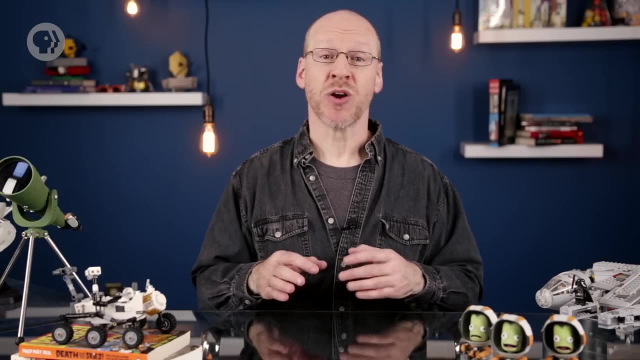 This was really bizarre. When a star explodes, it's a catastrophic event that should de-state any of the subspace planets in the universe. It's the last place anyone would have thought to find them. However, follow-up work quickly confirmed that the planets did indeed exist, and in 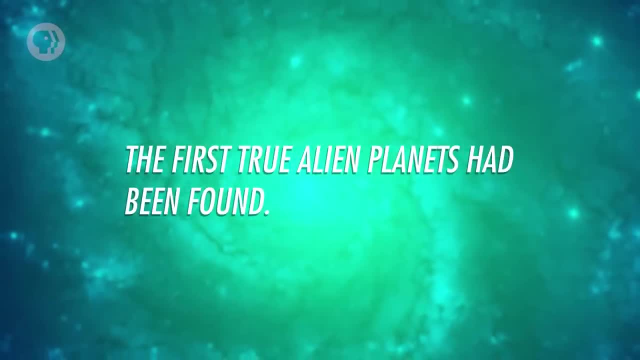 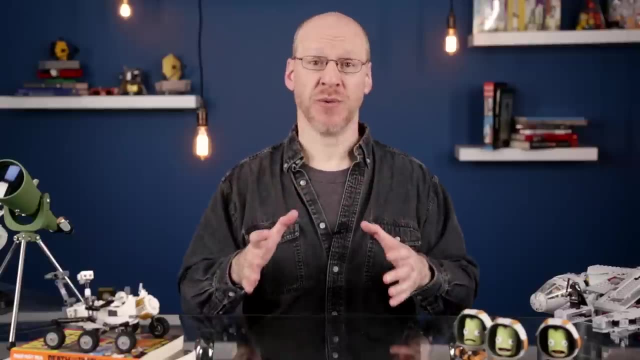 fact, a third one was found. a few years later, The first true alien planets had been found. Officially we call them exoplanets, which, you have to admit, is pretty cool. While this was an incredible discovery, it was still a little unsatisfying, For one thing. pulsars are really weird, and for another it looked like those planets may have formed around the pulsar after the supernova explosion, which is also a great thing, So it was, in fact, a big surprise from the material left over from the catastrophe. 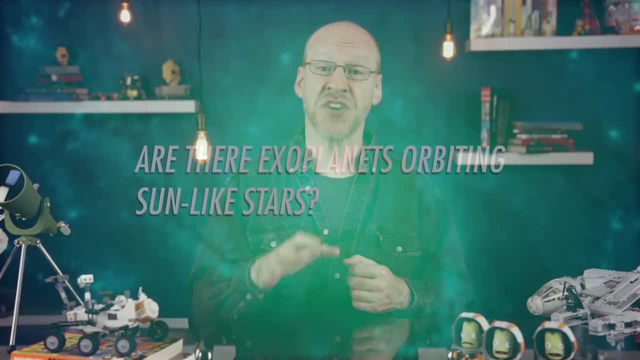 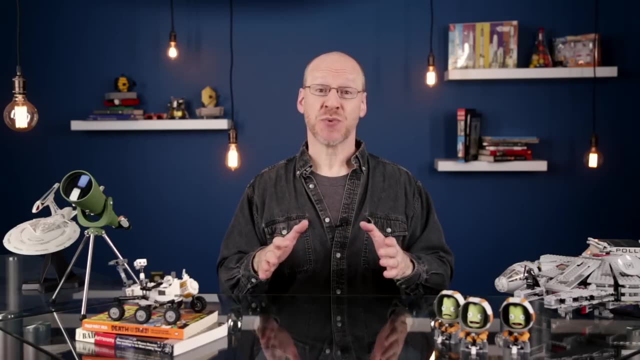 That's nothing at all like our own solar system, And that still left the question open: Are there exoplanets orbiting Sun-like stars? We didn't have to wait long to find out. In 1995, Swiss astronomers Michel Mayor and Didier Queloz made a big announcement. 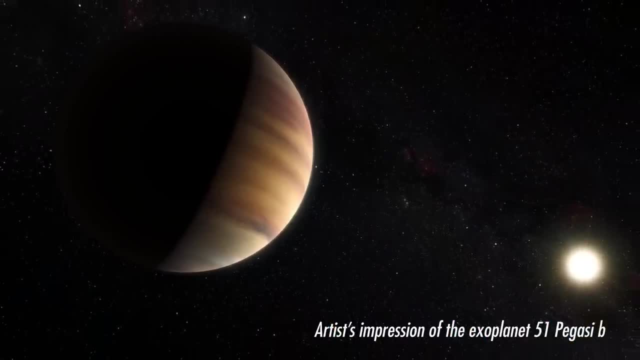 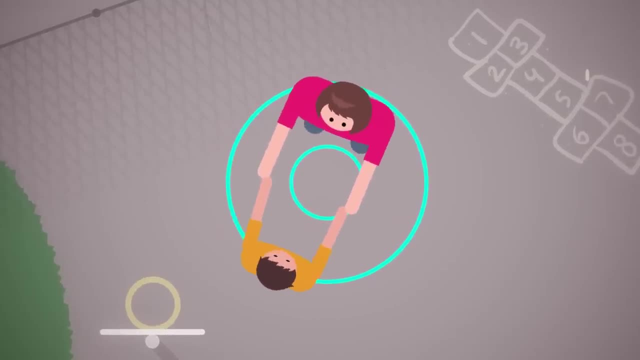 They had found a planet orbiting the star 51 Peg, a star very much like the Sun, just 50 light-years away. How did they do it? Well, remember those two kids holding hands and circling each other. Even though the wiggling back and forth of the star is too small to measure, that doesn't. 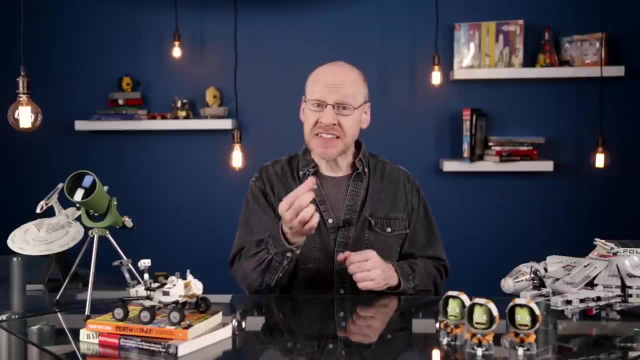 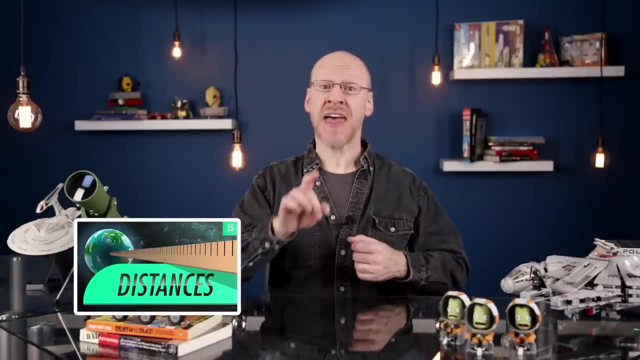 mean the effect is undetectable- As the host star of the exoplanet makes its little circle- sometimes it's headed toward us and sometimes away. That means that its light will undergo a Doppler shift and that can be detected. It's not a big shift and takes some pretty fancy equipment to see it, but it's measurable. 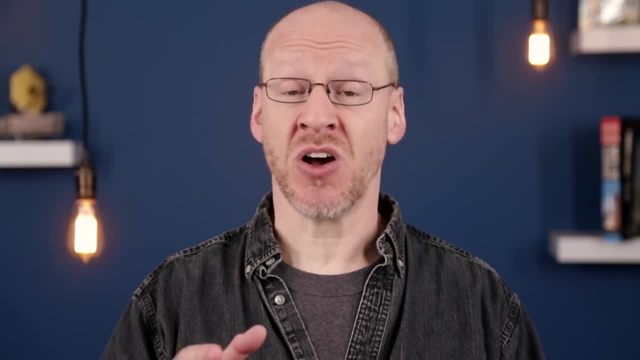 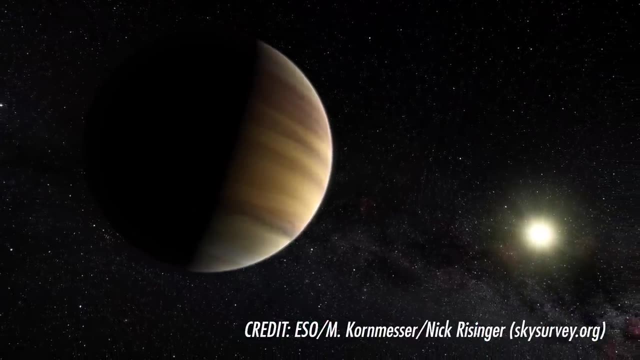 That's how Mayor and Queloz found their planet, And the planet they found, called 51 Peg B, is weird. For one thing, the orbital period turns out to be just a little over 4.5 million years away, That's 4.23 days. 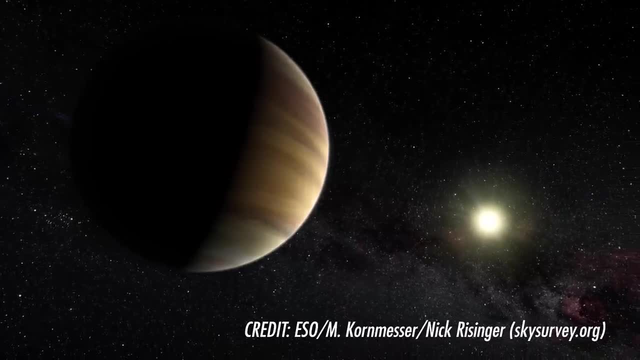 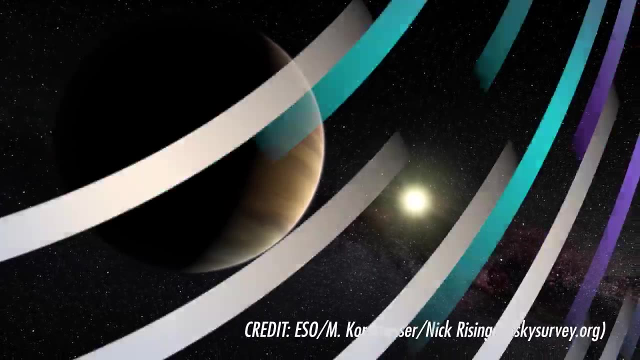 That's right. I said days. That means the planet is seriously close to its parent star, just 8 million kilometers out. Compare that to Mercury, which on average, is 55 million kilometers from the Sun. Not only that, but the amount of Doppler shift in the star is related to the mass of the 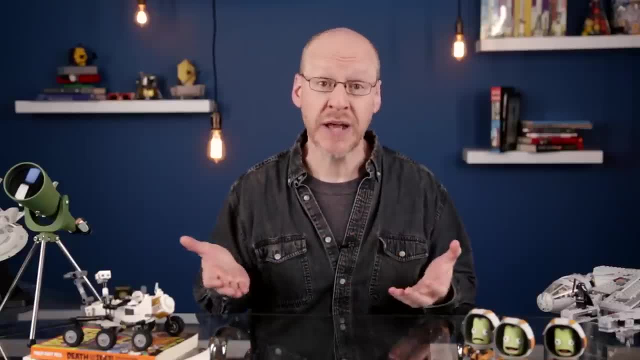 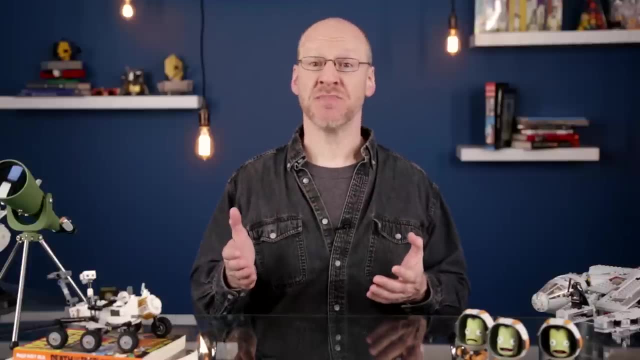 planet, A more massive planet, pulls harder on the star, making it move more quickly. They found the planet was at least half the mass of Jupiter, and probably more. That was a problem. According to planetary formation models, that wasn't possible. 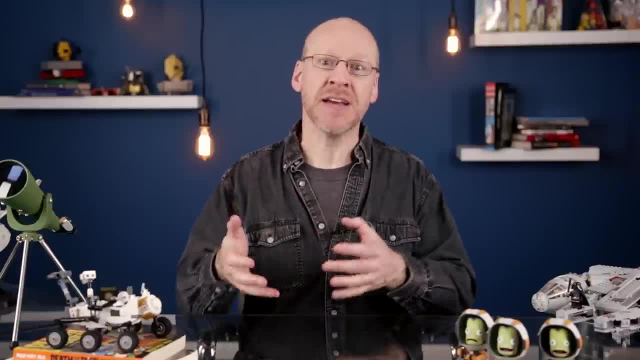 You wouldn't be able to see it. You wouldn't be able to see it. You can't form a planet that big, that close to a star. Well, it turns out, the models are probably right: The planet didn't form that close. It probably formed farther out, just like Jupiter did, And like Jupiter it then moved, migrated inward toward the star as it interacted with the disk of planet-forming material around the star In our solar system. Jupiter didn't get very far in its inward motion. It's thought that interactions with Saturn put the brakes on that and pulled Jupiter out to where it is now. Apparently, 51 Peg B didn't have its own version of Saturn pulling it out. It was a very small planet. There was nothing on it. 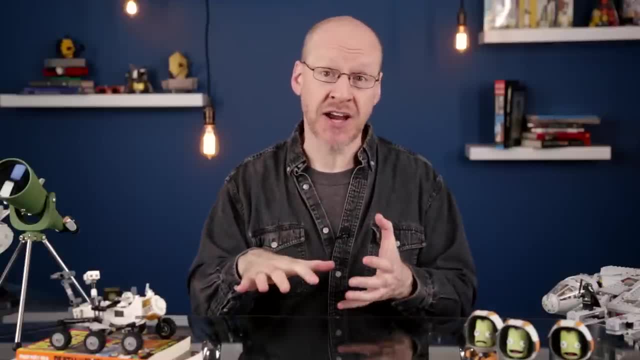 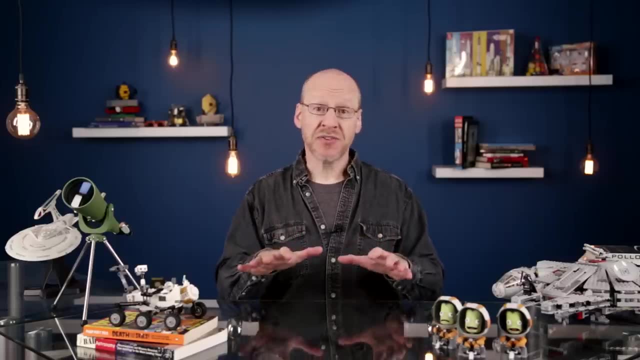 Its inward spiral continued until it ran out of disk material to interact with, which was very close indeed to the star We call planets like that hot Jupiters. Once 51 Peg B was found, other teams began looking for short-period planets, and within 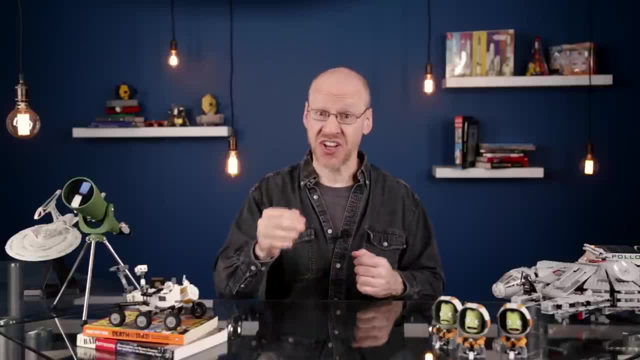 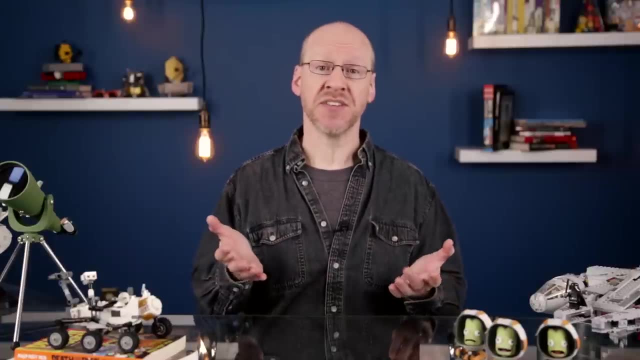 a few years several more had been found, many of them hot Jupiters, just like 51 Peg B. Now, mind you, at first there was a lot of doubt and skepticism in the community about these exoplanet discoveries. A lot of other phenomena could masquerade as planets, like star spots, pulsating star. 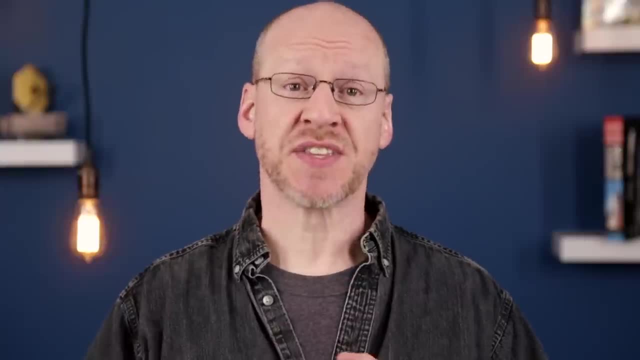 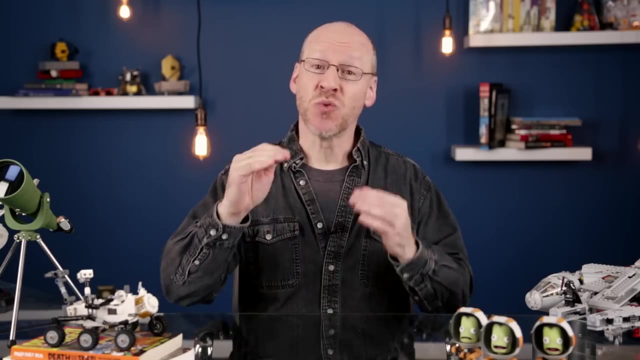 stars or background stars, messing up the measurements? Scientists discussed these possibilities vociferously as well. they should. Science is all about not fooling ourselves. A good scientist wants other scientists to try to poke holes in their ideas. It's disappointing to be wrong, but if we are, we want to know. 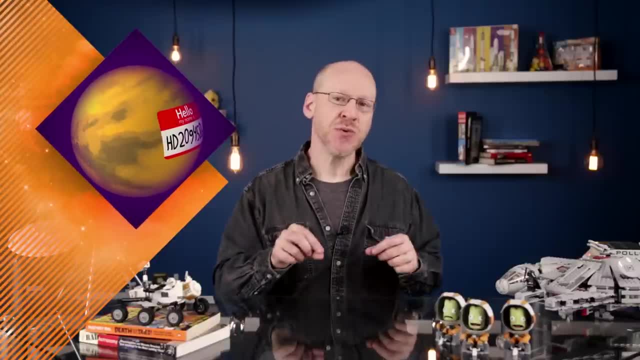 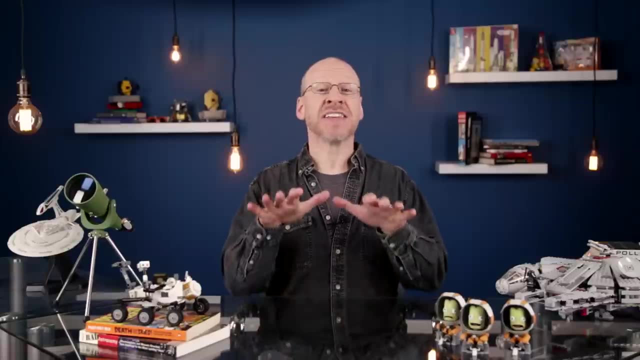 That all changed in 1999.. A planet called HD 209458 b had been discovered on a very short orbit around its star, taking just 3.5 days, As luck would have it. from Earth, we see the planet Jupiter. 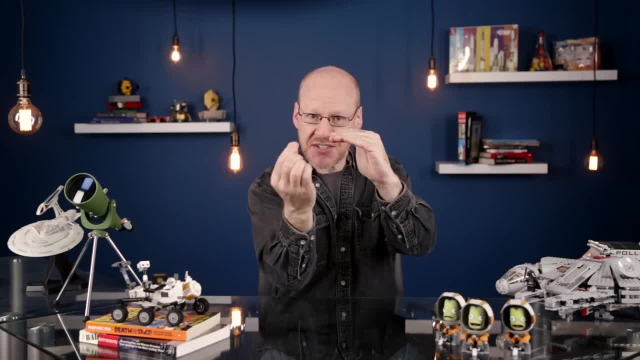 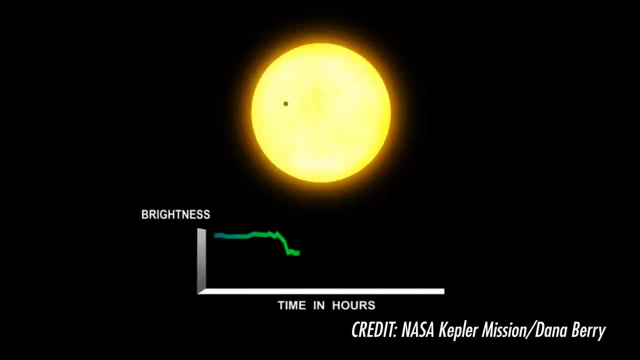 The planets orbit edge-on. That means once per orbit it passes directly in front of its star. This event is called a transit, and when the planet transits the star it blocks a little bit of the star's light And that means we can detect a dip in the star's brightness. 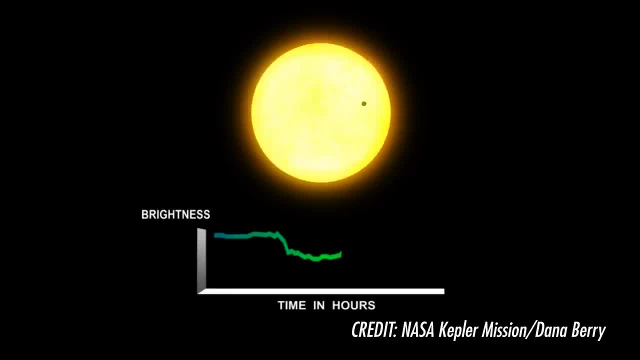 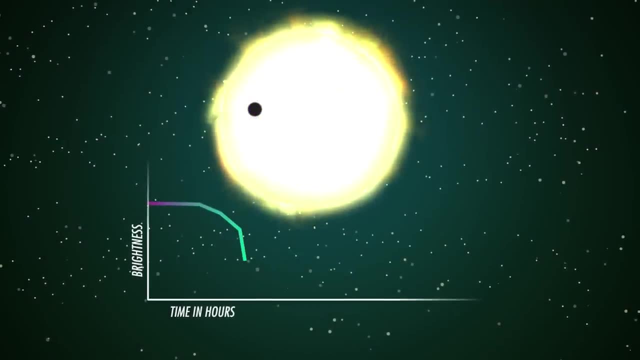 And sure enough that dip was found. HD 209458 b was the first independent confirmation of an exoplanet, and pretty much everyone was on the bandwagon after that. The beauty of transiting exoplanets is that the amount of starlight blocked tells you. 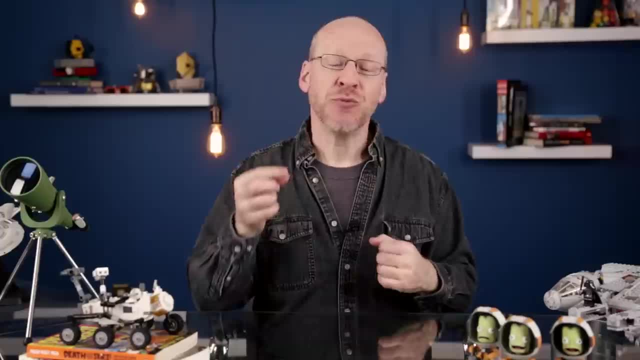 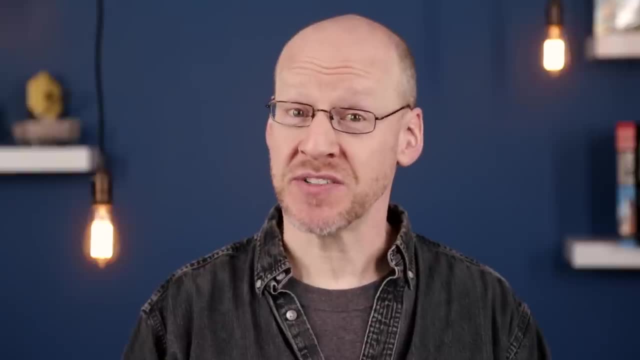 how big the planet is. A big planet blocks more light. If we know the planet's mass from the star's Doppler shift, we can use the planet's size to calculate its density. This is important. A gas giant like Jupiter has a low density and a rocky, metallic planet like Earth has. 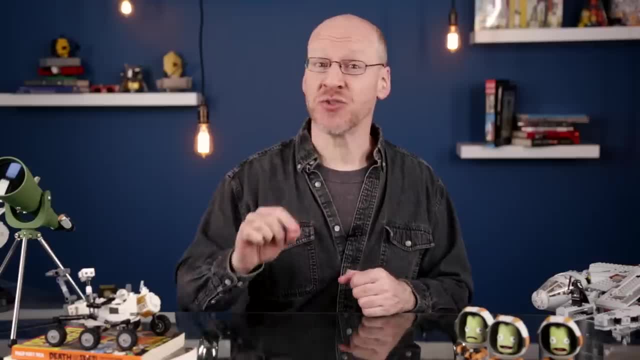 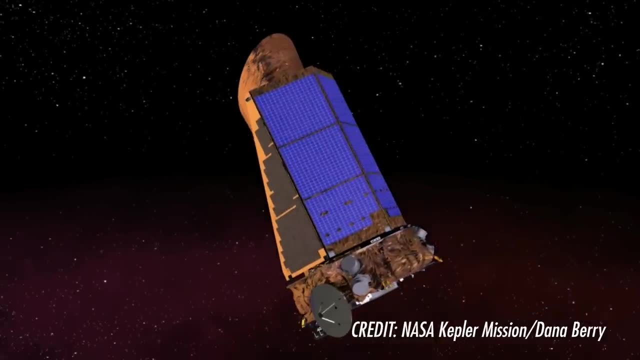 a very high density. Without even being able to see the planet directly, we can already start to determine what it's like physically. In 2009,, NASA launched a space-based telescope named Kepler, designed specifically to stare at 150,000 stars. 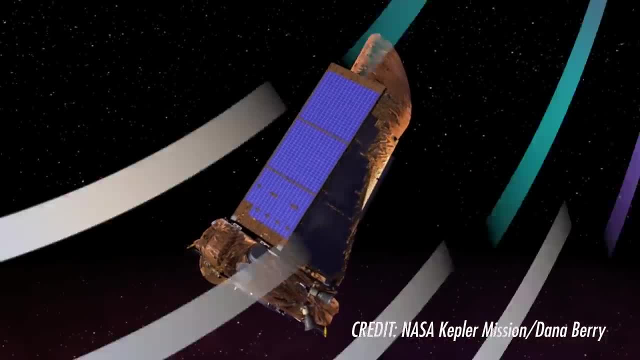 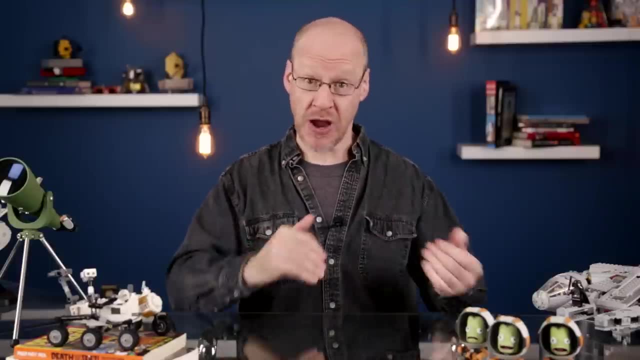 The telescope's light indicated exoplanet transits And, oh my, did it work. By early 2015, Kepler found its 1,000th confirmed exoplanet And there are 500 more confirmed from ground-based telescopes. 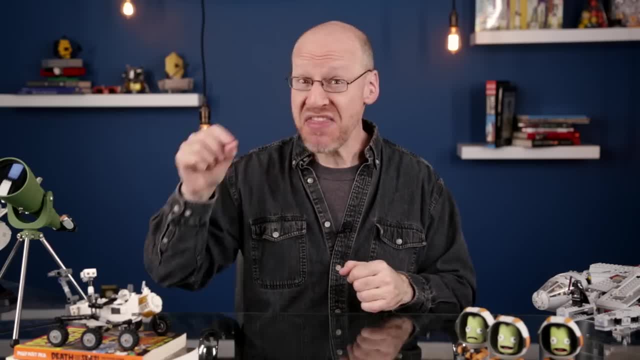 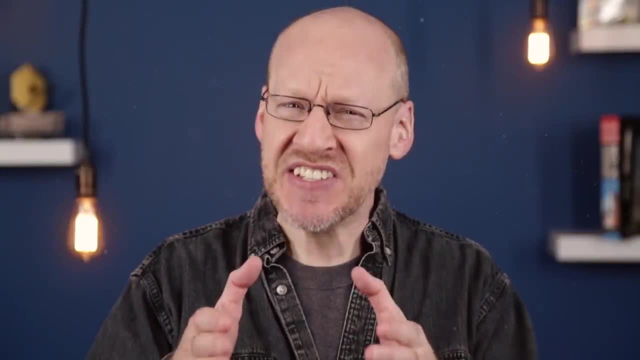 That's more than 1,500 planets, and we have well over 3,000 more candidates from Kepler awaiting confirmation. All these planets have been found using indirect methods. What about actually seeing them, getting photographs of them? That's hard because planets are so faint. But it's not impossible. In 2014, the NASA Space Telescope was discovered. In 2004, the first picture of an exoplanet was released: 2M1207b, a planet with five times the mass of Jupiter. 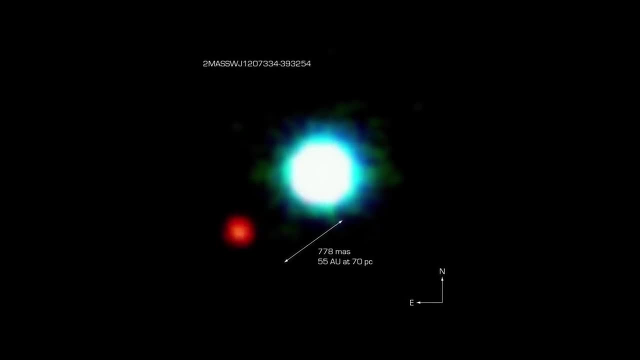 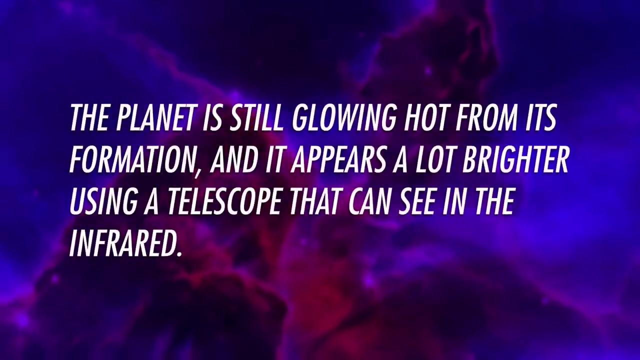 It orbits a brown dwarf, a peculiar kind of low-mass star that we'll learn more about in a future episode. It's a young system, which makes it easier to see. The planet is still glowing hot from its formation and it appears a lot brighter using a telescope. 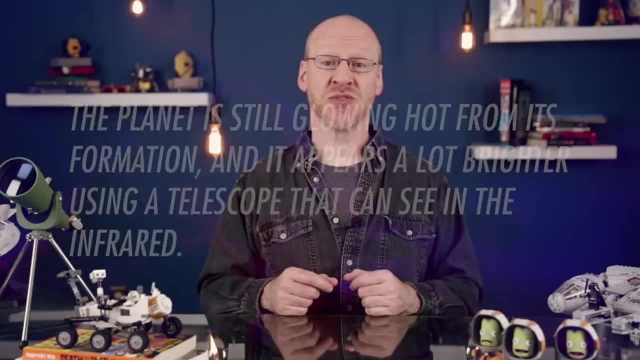 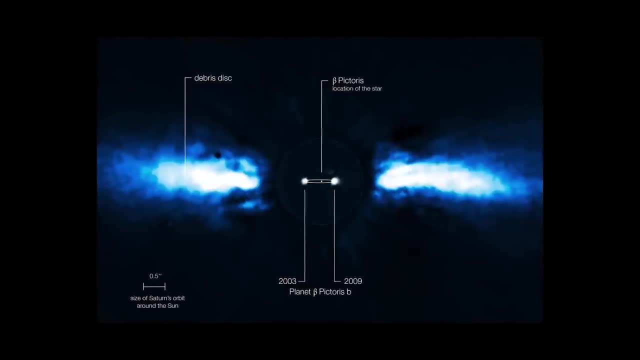 that can see in the infrared. About a dozen other planets have been seen this way too. My favorite is the planet orbiting the star Beta Pictoris. It has seven times the mass of Jupiter. It orbits the star in about 20 years and we've actually seen it move. 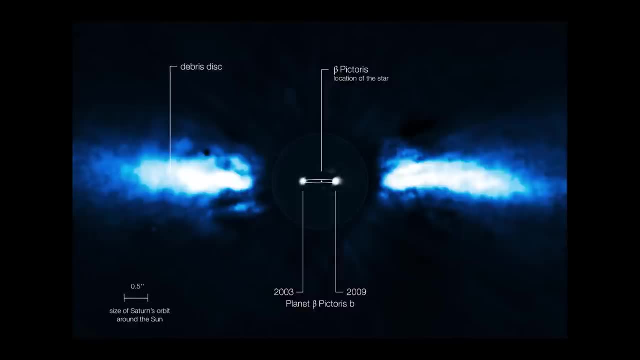 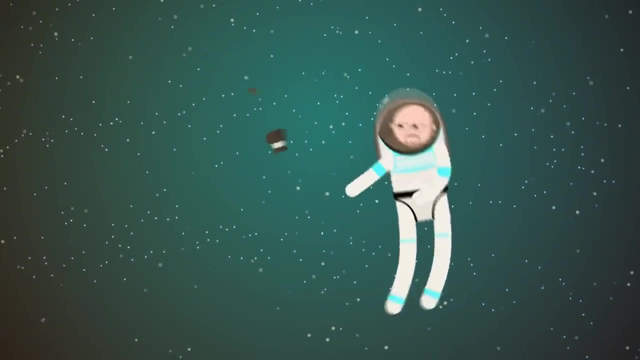 Images taken a few years apart actually show the planet in different positions around the star, confirming its orbital motion. That is incredible. Taking photos of these planets is still a daunting task, which is why so few have been seen, But we're getting better at this and as new technology comes along, we'll get more. 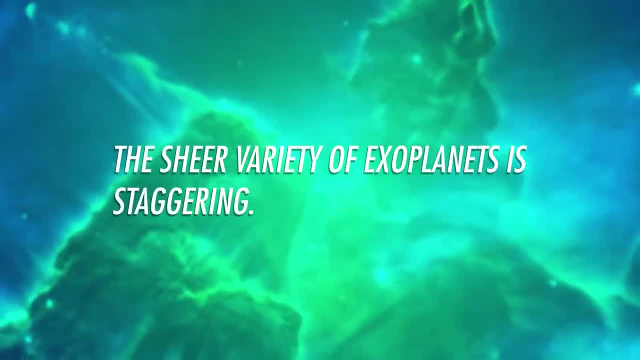 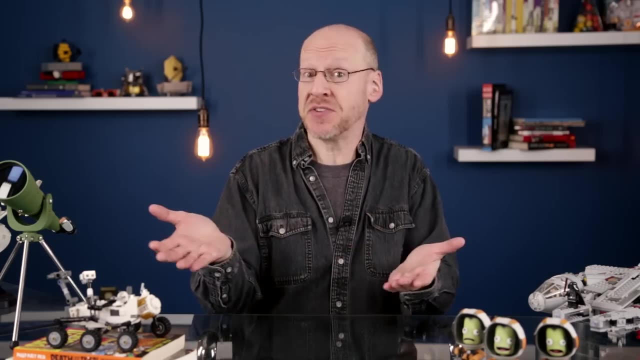 pictures of exoplanets and learn even more about them. The sheer variety of exoplanets is staggering. Hot Jupiters are the easiest to find because they're massive and massive. But they're not just exoplanets: They can run fast, making their signal easier to detect. 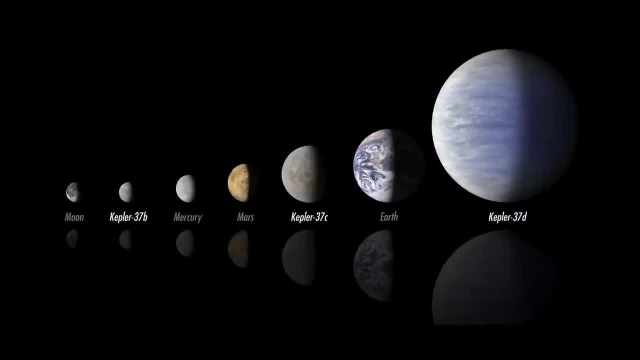 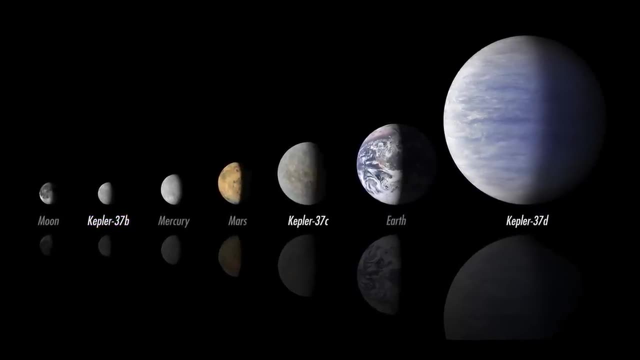 But as the techniques have improved, planets of lower mass have been seen. The smallest exoplanet found is smaller than Mercury and not much bigger than Earth's moon. We've seen planets bigger than Earth but smaller than Neptune, called super-Earths. About 500 multiple-planet systems have been found too, including one with seven planets. We've found them around every kind of star too. Exoplanets have been detected around stars like the Sun, as well as tiny cool red dwarfs. hot massive blue stars And even red giants stars nearing the ends of their lives. One exoplanet system announced in 2015 is incredibly old. The host star is 11 billion years old. When our solar system was just beginning to form, these planets were already over 6 billion. years old — older than our solar system is now. We've even seen planets orbiting binary stars, making Star Wars seem a lot closer to home than being in a galaxy far, far away. We've seen so many exoplanets now that we can extrapolate a bit and get some numbers. 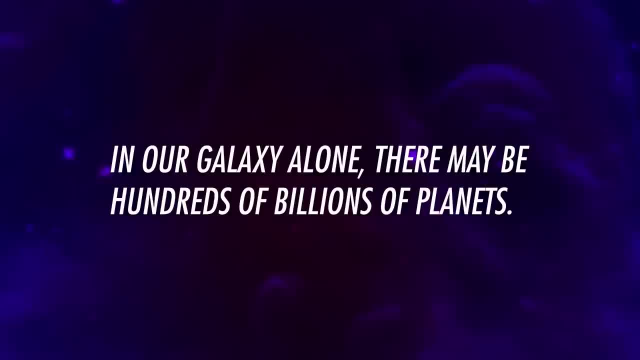 We've even seen planets orbiting binary stars, making Star Wars seem a lot closer to home than being in a galaxy far, far away. We've seen so many exoplanets. now that we can extrapolate a bit and get some numbers, The results are staggering. 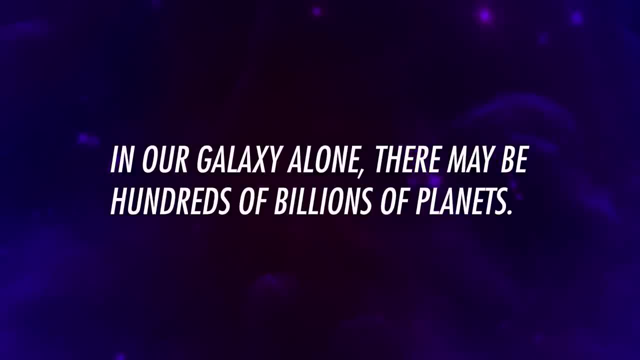 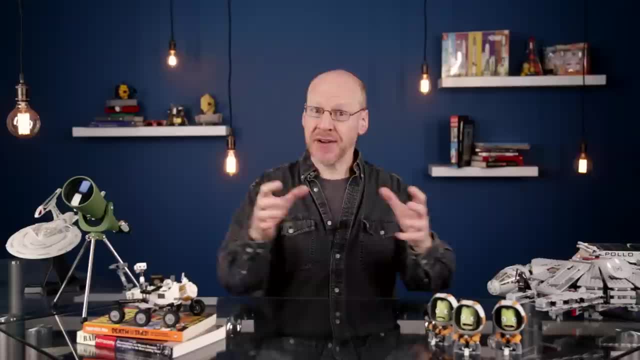 In our galaxy alone, there may be hundreds of billions of planets. In fact, planets may outnumber stars in the sky. Now, if we've seen planets as big as Jupiter and as small as Mercury, then we must have seen planets around the same size as Earth, right? Yes, Yes, we have. We've actually found hundreds of them so far. It looks like making planets the same size as ours is pretty easy for stars to do, But Earth-sized is one thing, Earth-like is another. How many of these planets might actually be habitable? that is at the right distance. 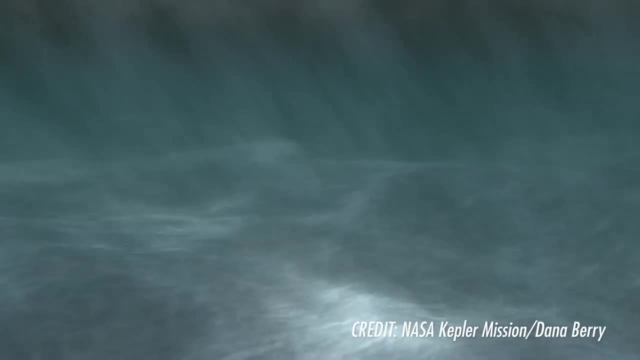 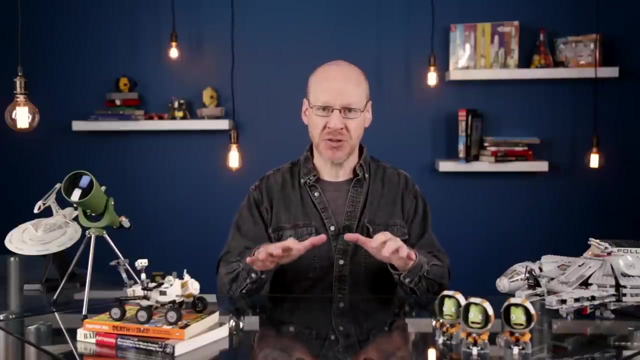 from their star to have Earth-like conditions where liquid water could exist on their surface. We're not sure, but from what we've seen so far, it looks like the galaxy may have more than 10 billion Earth-like planets, Ten billion. 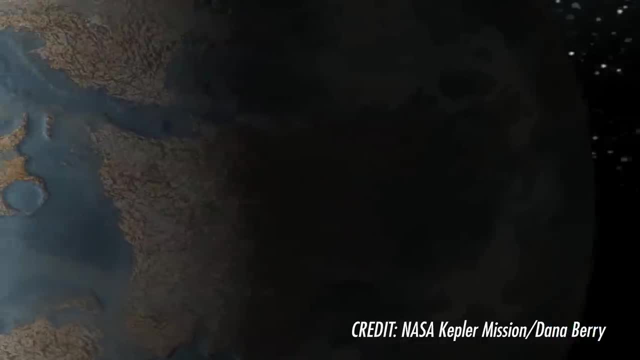 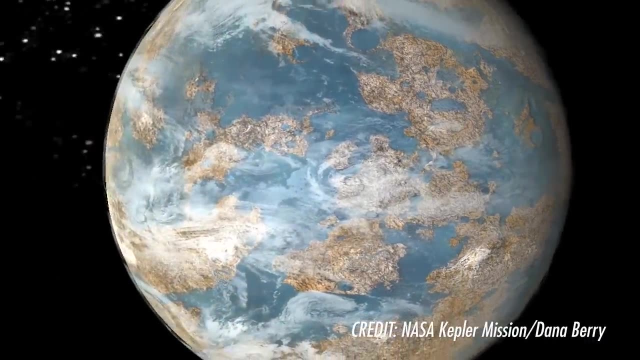 And maybe a lot more than that. Now I want to be careful here. We don't know what kind of atmospheres these planets will have or what they're composed of. Do the planets have magnetic fields strong enough to prevent solar wind from eroding? 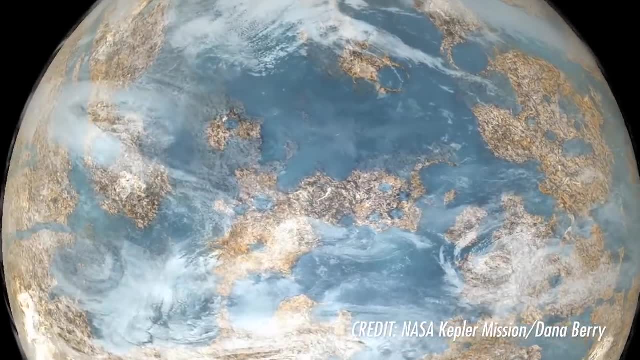 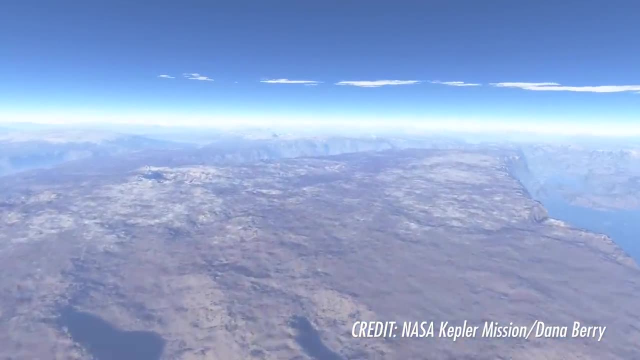 away their atmosphere? Do they even have an atmosphere, let alone liquid water? We don't know, But still there are a lot of planets out there. There could very well be a twin of Earth orbiting a star not too far away.